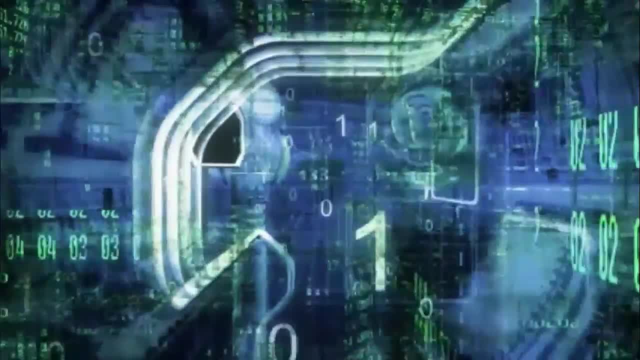 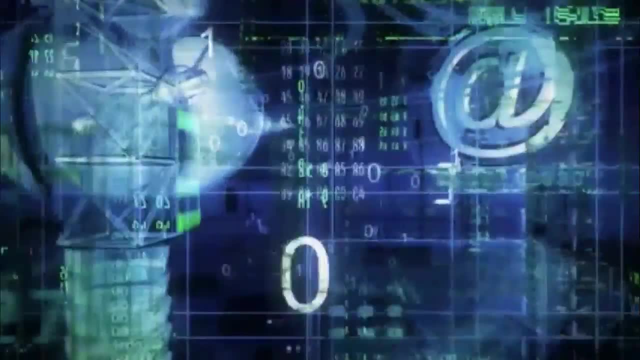 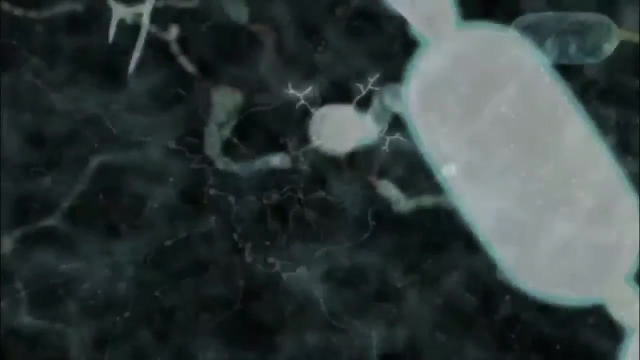 Visual information must first be processed to become useful. it must be coded and assimilated, it must be compared with prior information and it has to be analyzed, just like a computer does. Visual information processing is mistakenly believed to be only located in a small part of the brain. 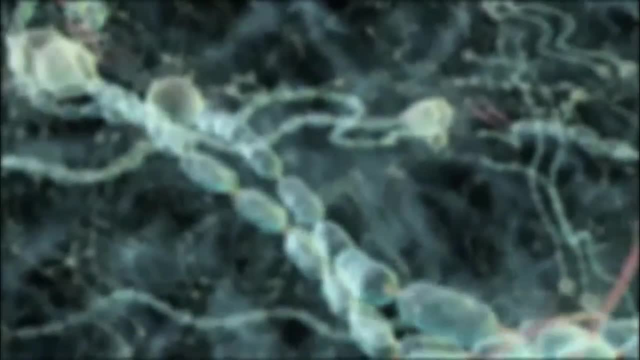 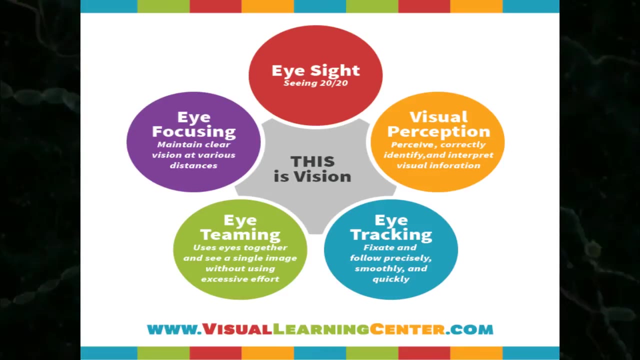 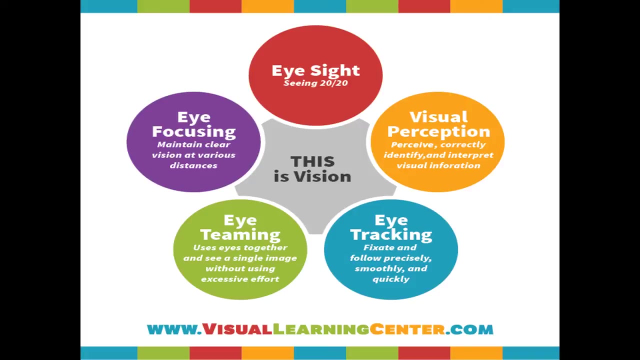 In fact, the processing of visual information takes place in over 80% of the brain, and this processing is influenced by other sensory information. A complete developmental vision exam starts with determining if a child has clear eyesight. If they do, we must determine if they have good focusing skills. 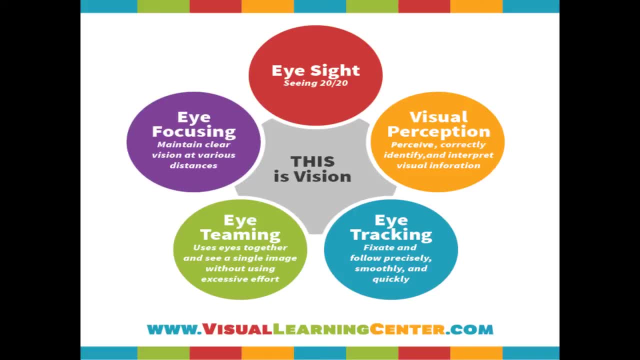 Can they sustain that clear eyesight for an extended period of time And can they shift their focus back and forth from the front of the classroom to their desk? Eye-teaming is the ability to use the eyes in a corner, To use the eyes in a coordinated fashion, and if so, can the child do so long enough to read many pages in their textbook? 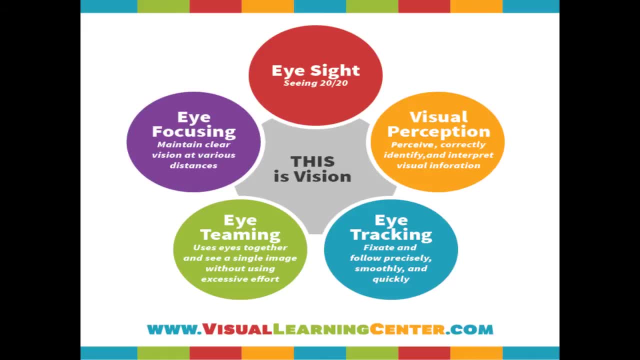 Eye-tracking is the specific eye movement used while reading, and this is rarely tested for in routine eye exams that check for eyeglasses or the health of the eye. Once visual information has been gathered by the eyes, it must then be processed. Visual, perceptual or visual processing skills allow us to decode and then act on what we see. 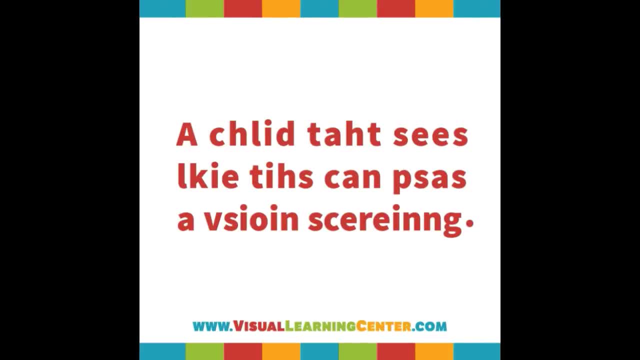 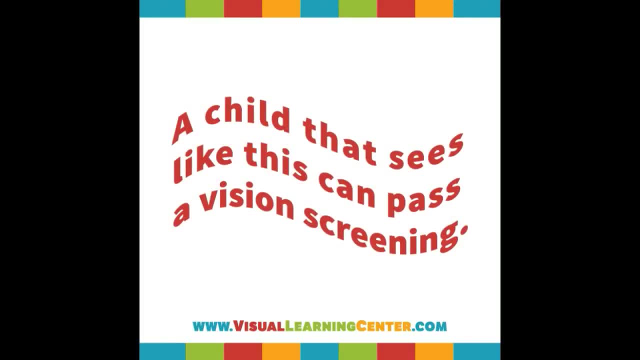 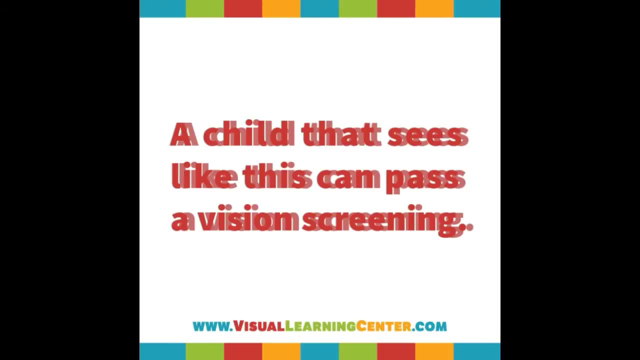 Many poor readers struggle with letter reversals Or problems with eye-teaming and tracking, which makes words and lines wavy or appear to move around on the page, And some children will notice the print on a page will get blurry after reading for just a few minutes. 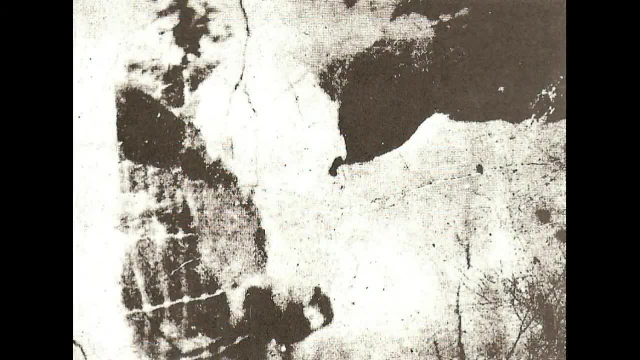 If you have good eyesight, you can see this picture of a familiar object clearly. So what is it? But visual processing skills allow you to derive meaning from what your eyes see. Do you see it now? Do you see it now? Do you see it now?